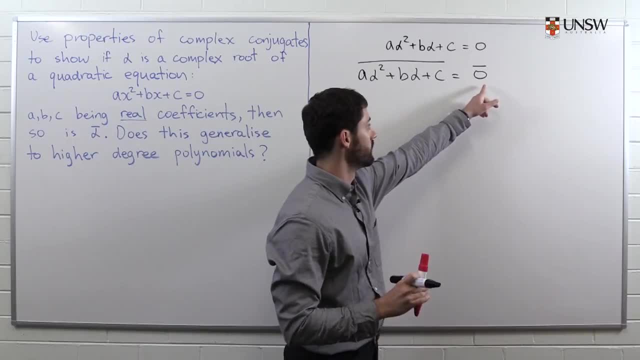 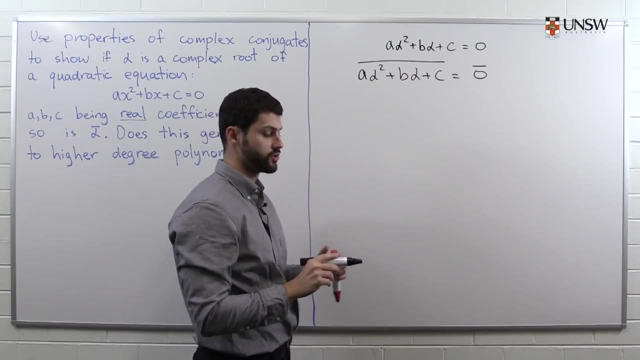 conjugates to simplify. simplify this. So, first of all, the conjugate of 0 is 0. The other property we're going to use is, if we have sums of complex numbers and we take the conjugates, we can first take. 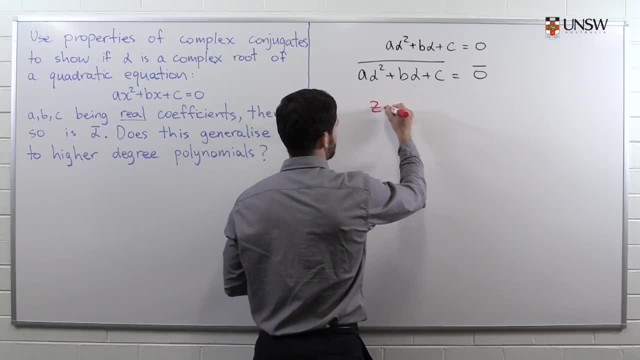 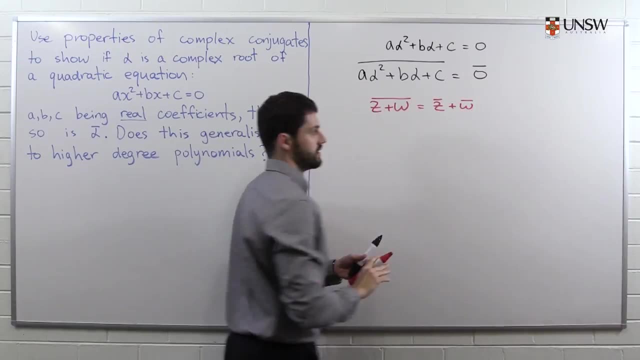 the conjugates and then take the sum. So in particular, if we have two complex numbers- z and w- and we take the conjugate, it's the same as first taking the conjugates and then adding them together. So if we apply this formula to this particular situation, we get: 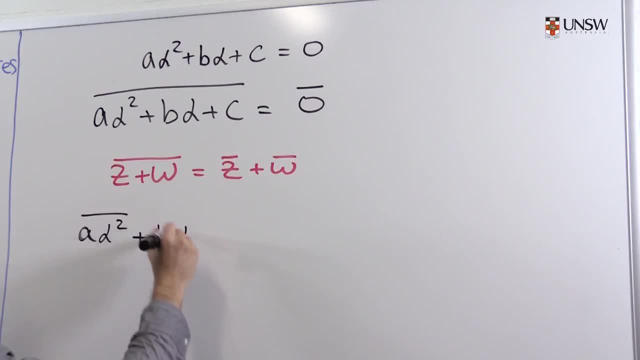 a alpha squared conjugate plus b alpha conjugate plus c conjugate and, as I said, the conjugate of 0 is 0, so we just get 0.. Okay, here we have a product of numbers, So we're going. 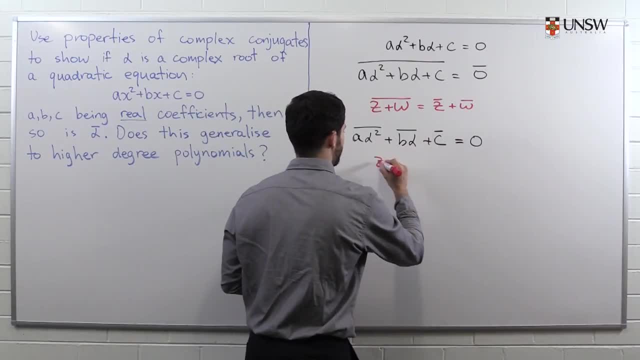 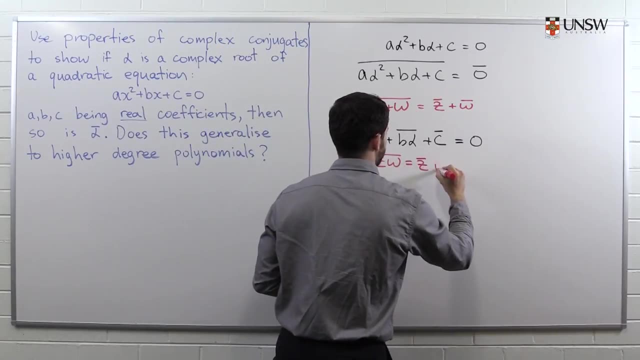 to use another property of complex conjugates, which states that if we have a product of two complex numbers and we need to take the conjugate again, we can just do it one at a time. So first take the conjugates and then take the product. So if we apply the 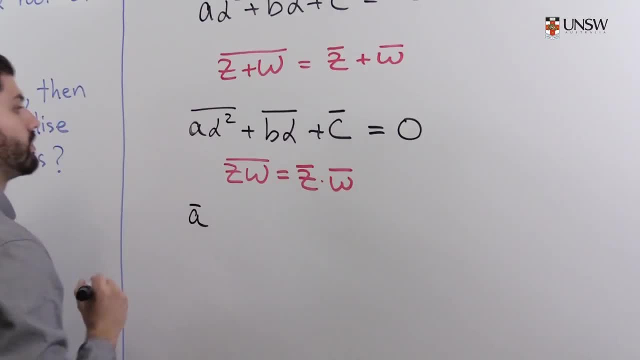 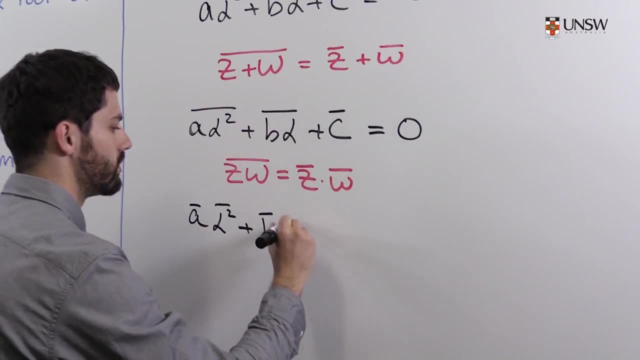 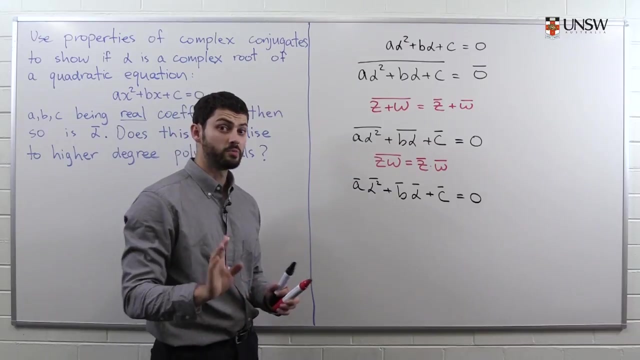 formula to this situation: we get: the conjugate of a multiplied by the conjugate of alpha, squared, plus the conjugate of b multiplied by the conjugate of alpha, plus the conjugate of c, equals to 0.. Okay, and now comes probably the most important part, and that's the fact. 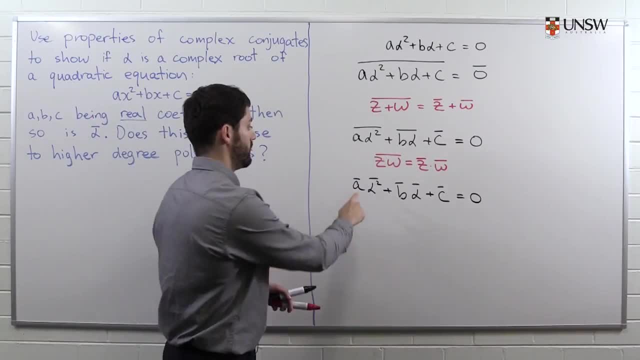 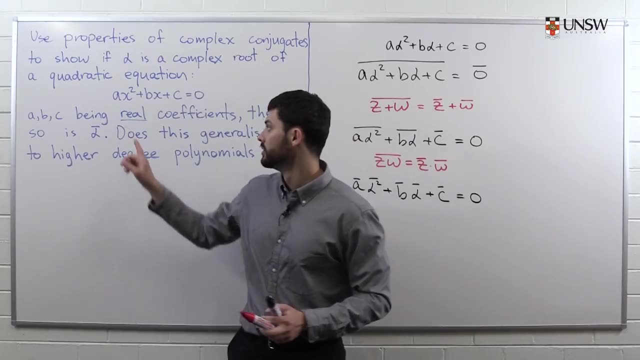 that because a, b and c are real, the conjugate of a, the conjugate of b and the conjugate of c is just equal to a, b and c, And this is only true because they're real numbers. In fact, this result is false if 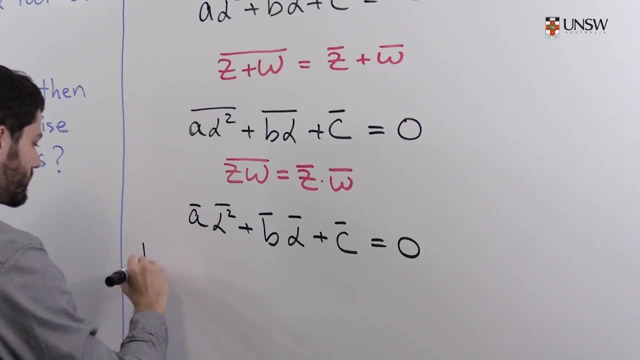 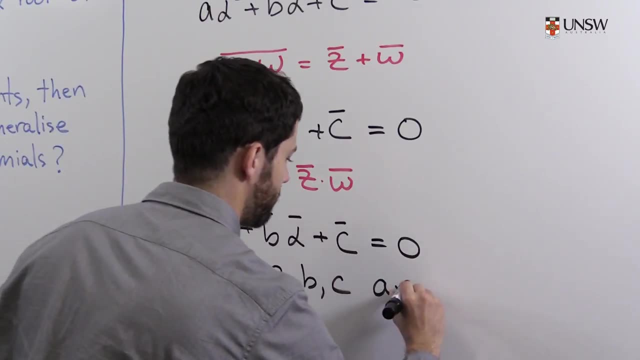 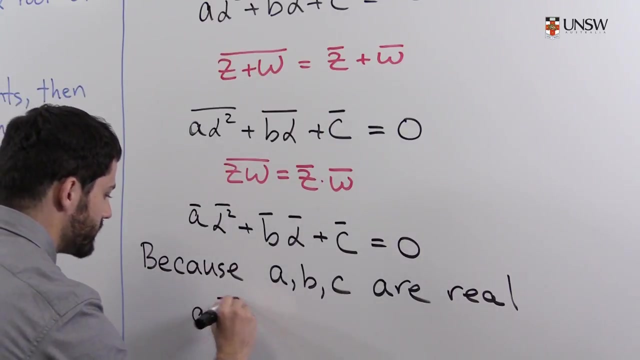 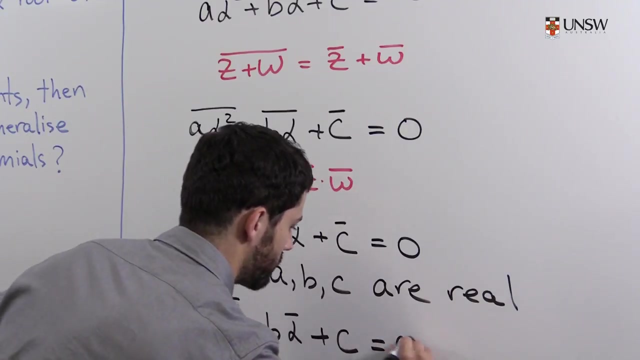 we don't assume that a, b and c are real. Okay, so because a, b, c are real, we can now say that this is the same as a conjugate of alpha squared plus b. conjugate of alpha plus c equals to 0.. 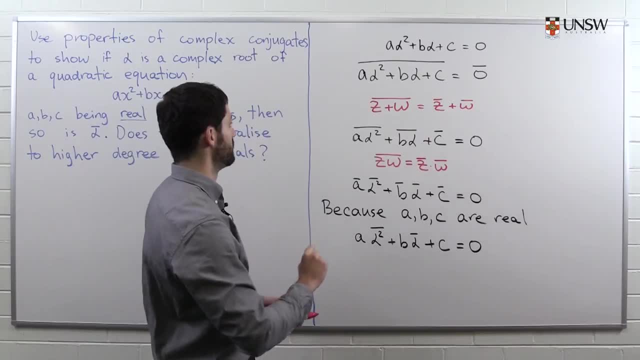 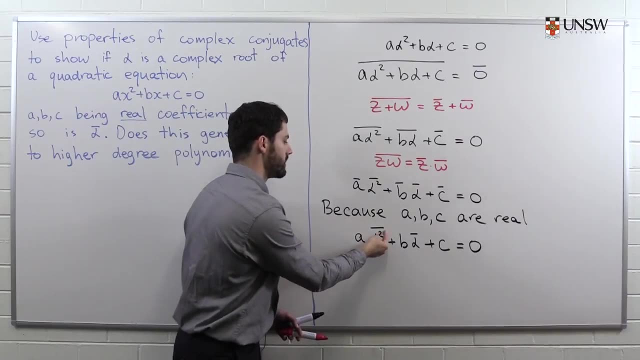 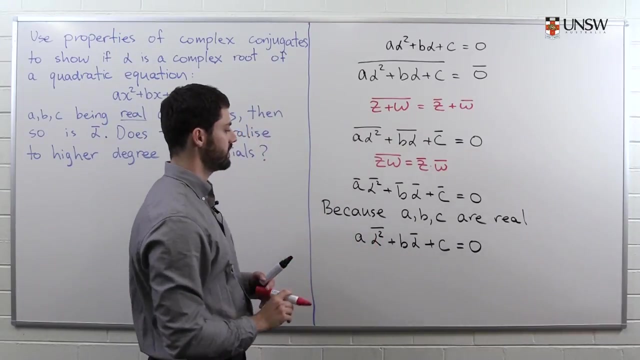 Okay, we're almost done. This is almost like substituting the conjugate of alpha into here, except here we have alpha squared conjugated and we need the other way around. We need to say we want to have the conjugate of alpha squared, but luckily again there is another. 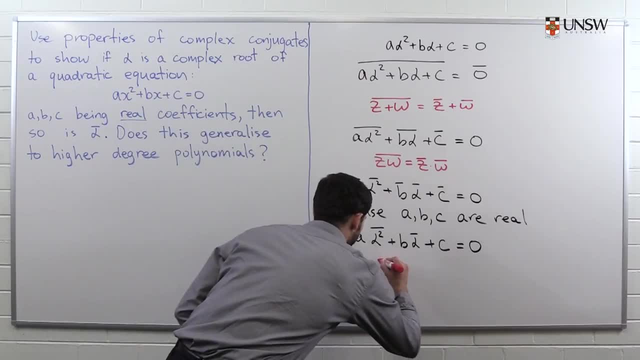 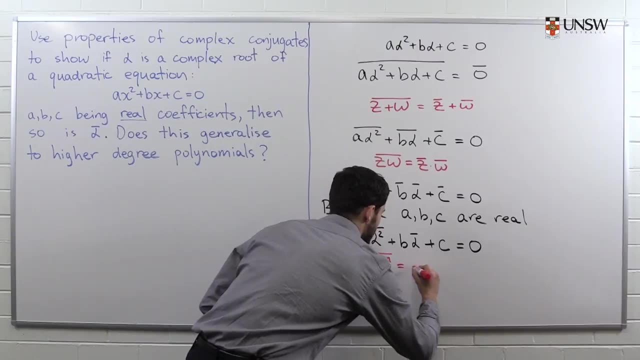 rule about complex numbers which we can use here, and that's the fact that if you take a complex number, raise it to some power and take the conjugate. that's exactly the same: you first conjugate and then raise it to this power. 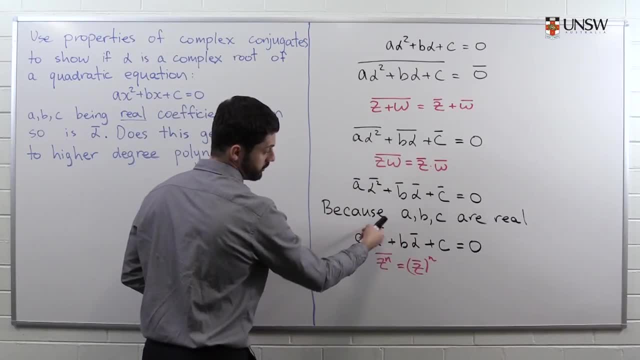 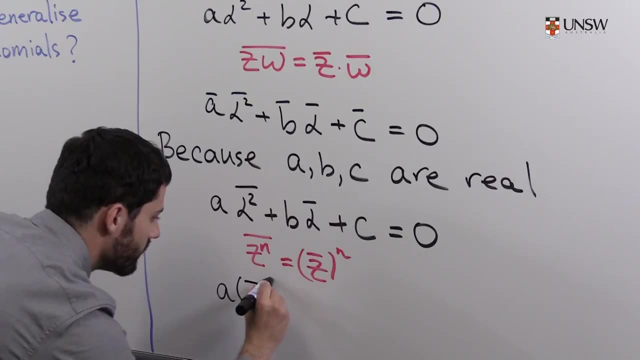 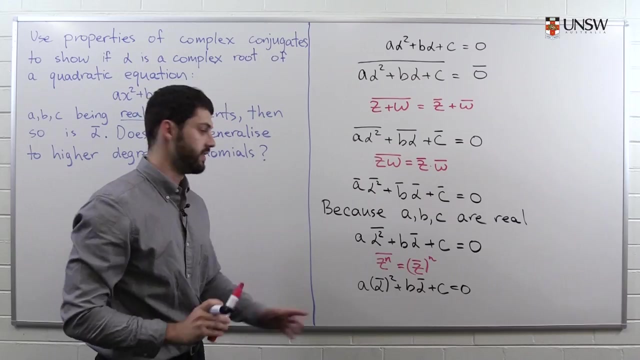 Okay, so now, if we apply this rule, we only need to apply it to this coefficient here. so then we get a conjugate of alpha squared plus b. conjugate of alpha plus c equals to zero, and that's precisely what we get if we substitute the conjugate of alpha instead. 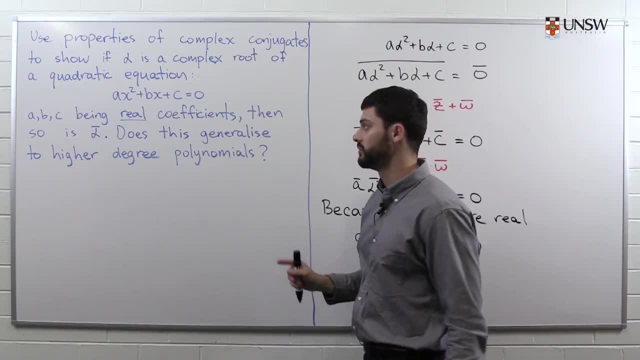 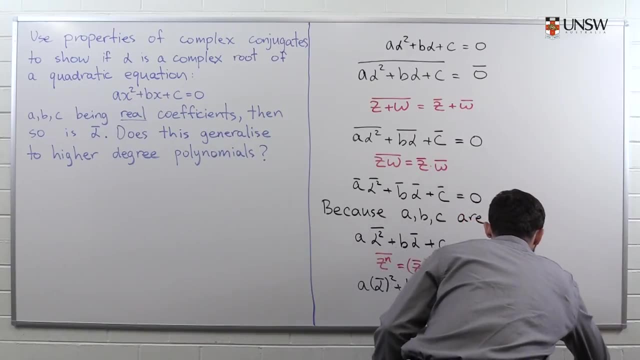 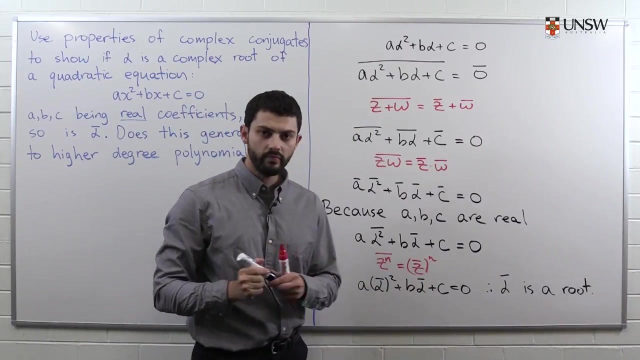 of x here instead of substituting alpha, which by definition means the conjugate of alpha is the root of this equation. So we can say now: therefore, alpha conjugate is a root. Okay. so the next part of the question asks: does this generalize to higher degree polynomials? 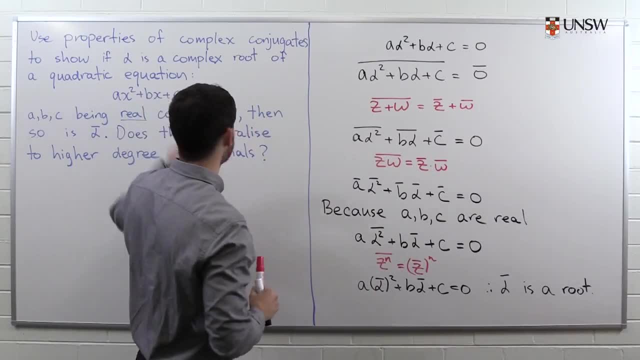 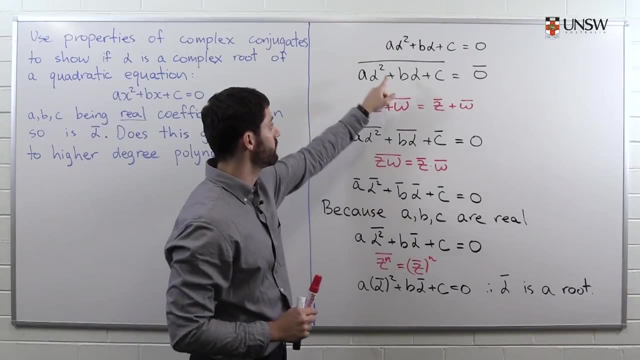 So was there anything special here that only worked because this was a 2?? And I hope you can see that. You can see that the answer is no. None of the rules here I used relied on the fact that this is a 2.. 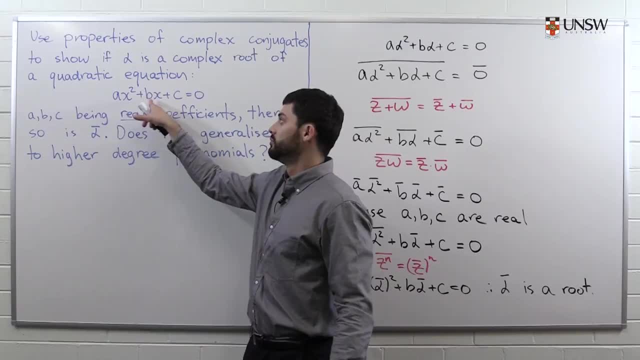 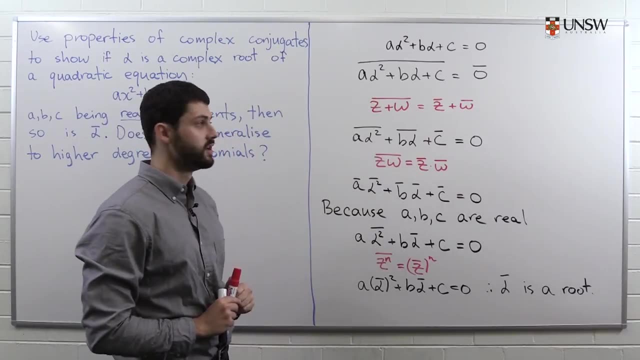 We could have easily had ax cubed plus bx squared plus cx plus d equals to zero, and this proof would have worked exactly the same. Nothing would have changed. We would have used exactly the same rules in exactly the same order and come to exactly. 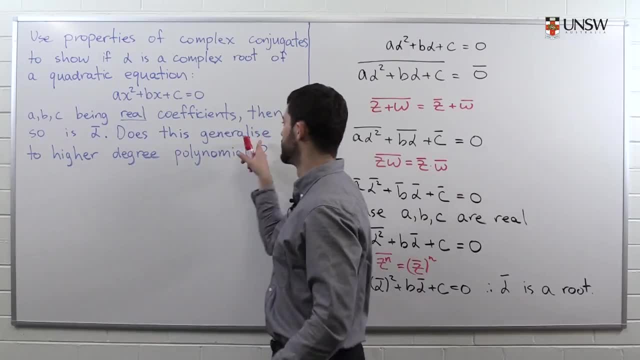 the same conclusion. So the answer to this question is: does this generalize? The answer is a big yes, Thank you.